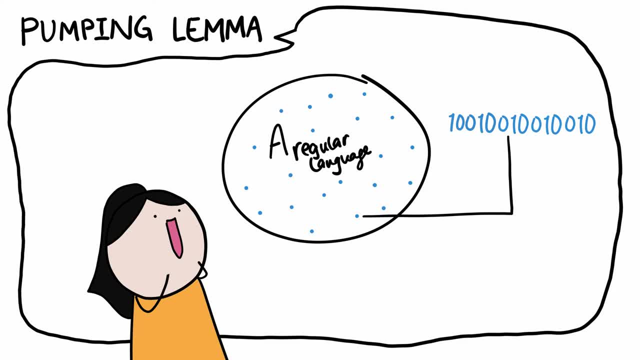 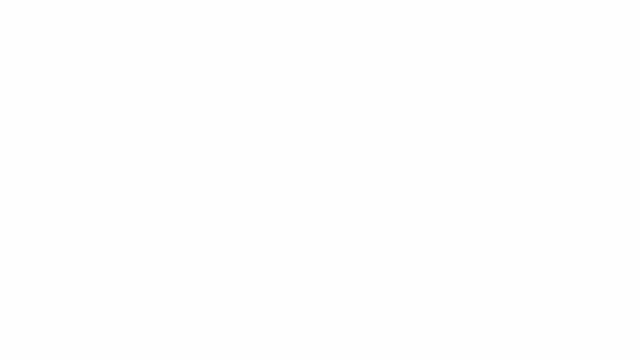 and, as usual, we'll try to provide some intuition for the concept instead of the technical details. So how exactly does the pumping lemma work? Let's take the regular language A that contains every string that ends with 11 and its DFA, as an example to understand the pumping lemma. 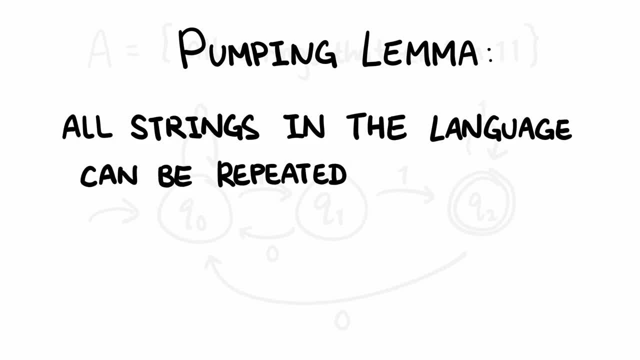 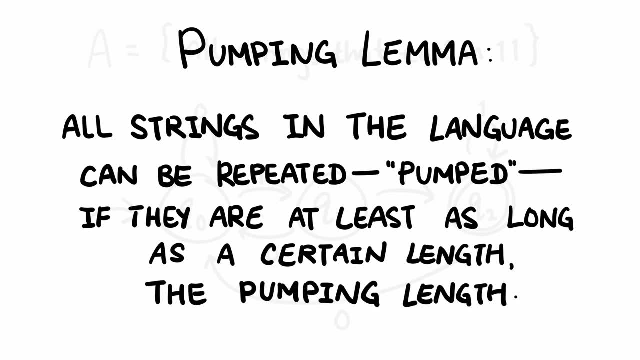 The pumping lemma states that all strings in the language can be repeated or pumped if they are at least as long as a certain length, which we call the pumping length. Let's call this pumping length P For our example. we can assign the pumping length. 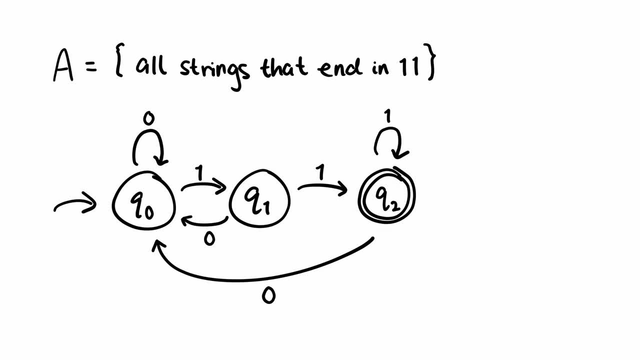 to be the number of states of A's DFA. So P will equal 3.. Now let's see how the machine runs on some strings in A that are at least length 3, such as 011, 1011, and 01111.. For all these strings there must have been at least one repeated state. 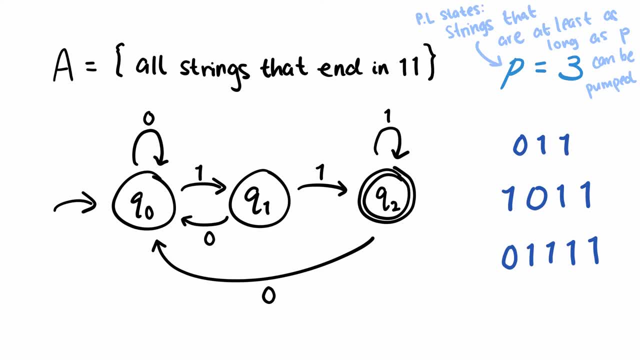 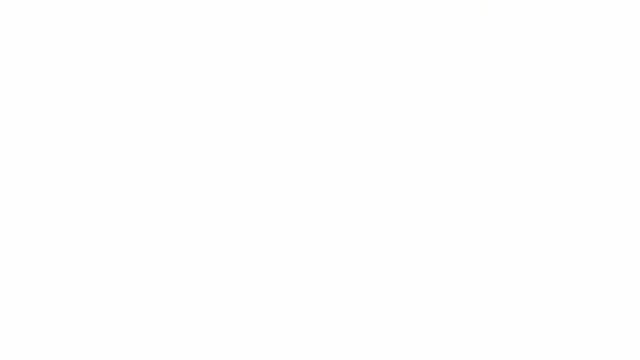 which can provide a section of the string being pumped. So, for 011, we revisited Q0 using the substring 0.. For 1011, the substring 10 took us between Q0 and Q1.. And for each of these substrings, the pumping lemma states that we can pump them as many times. 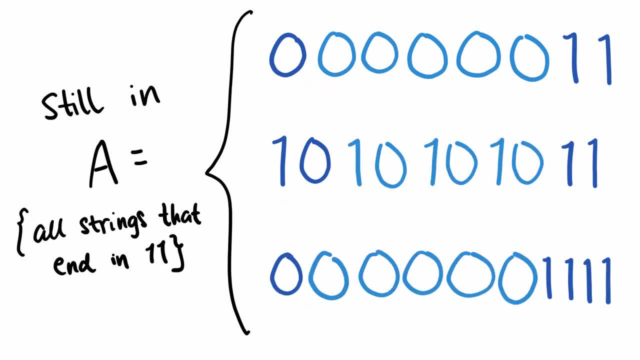 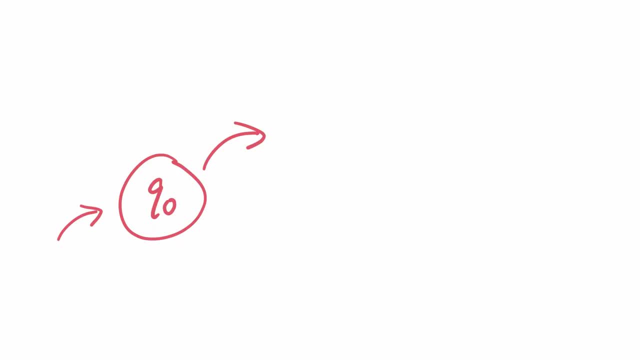 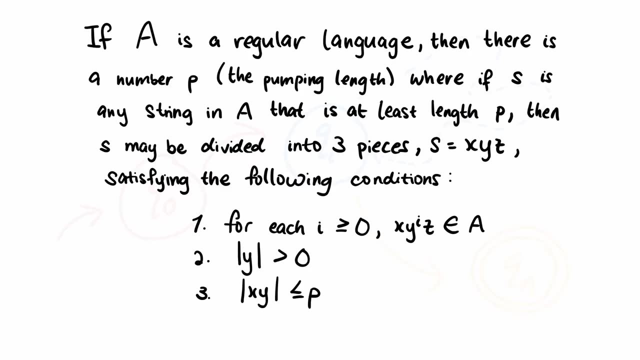 as we want, and the resulting string will still be in the language. Now notice how we can separate these strings into the part before pumping, the part being pumped and the part that takes us to the accept state, which, if you look at the formal statement of the 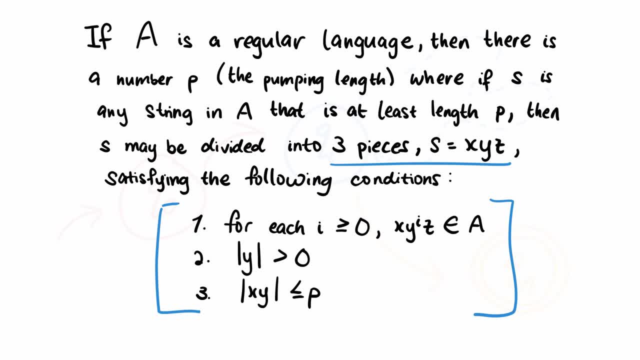 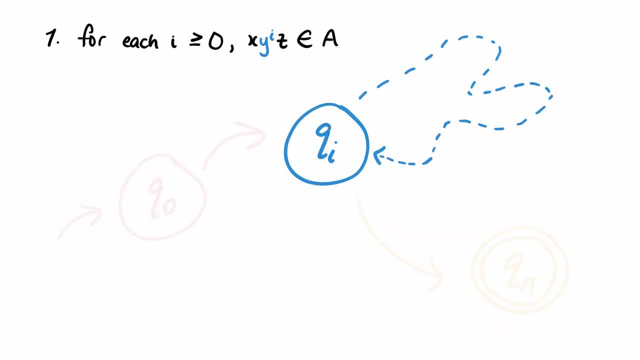 pumping lemma is what all this means. The following three points are just some more technical conditions. The first point says that for any string in the regular language there will be a part that can be pumped any number of times, which we call y. 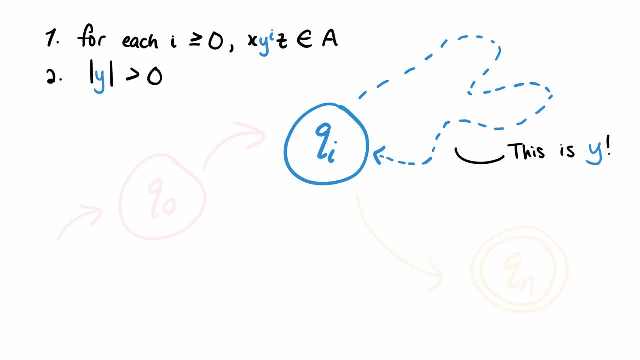 The second point says that the length of y has to be greater than 0,, which means we cannot pump the empty string. So if we look at each string as three parts- x, y, z- the part y being pumped cannot be empty, but x and z, which are the parts before and after the